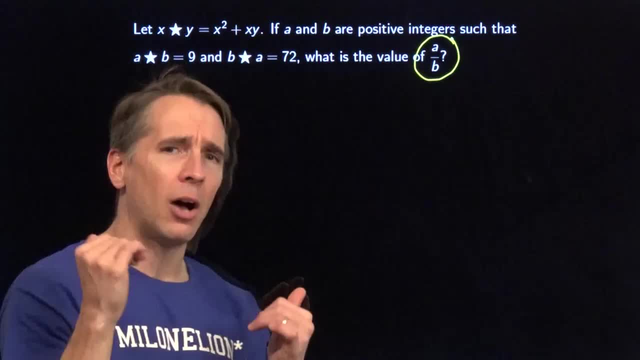 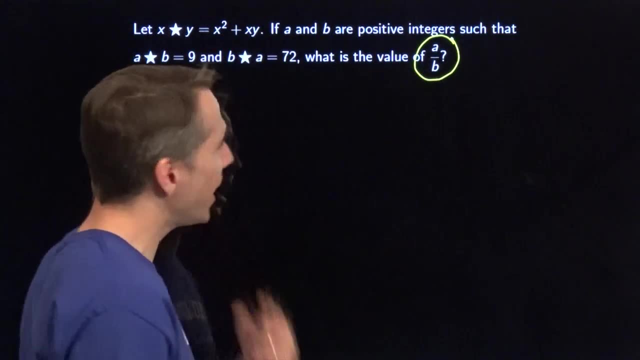 Alright, we're going to keep our eye on the ball. We're going to get to work here. We have to find stuff about a and b, And all we have are these weird equations with stars in them. But we know how to handle those stars. They tell us how to handle them right up there. 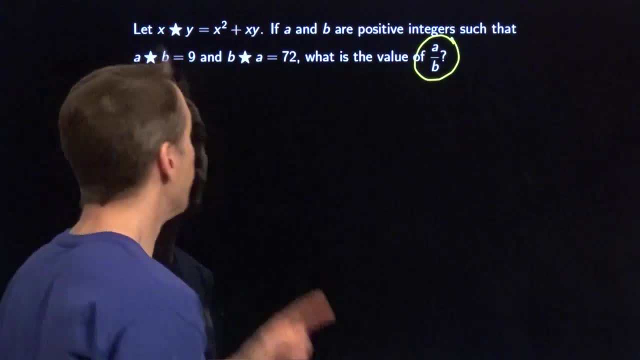 We take this a, star b and we use our definition. The a comes before the star, just like the x does in our definition. But we don't know how to handle those stars. They tell us how to handle them right up there, So we put the a where the x's are over here. 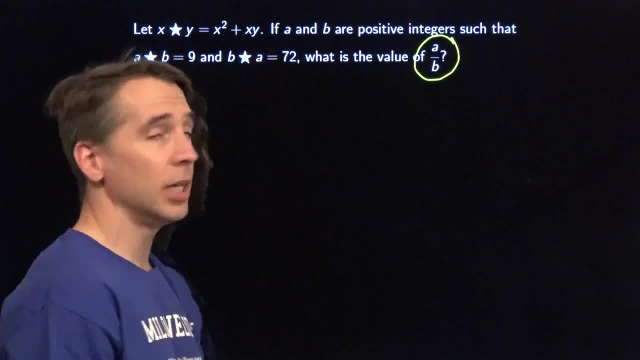 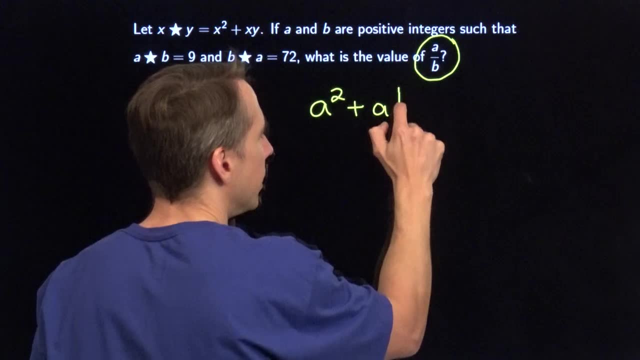 The b comes after the star, like the y does. b goes in for y, So a star b is a squared plus a times b, And we're told that that equals 9.. Then we do the same thing for this equation, right here. 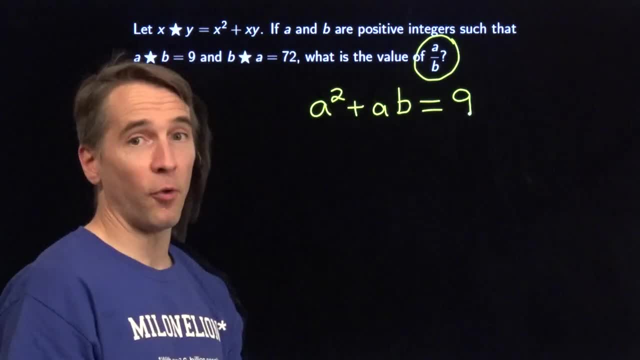 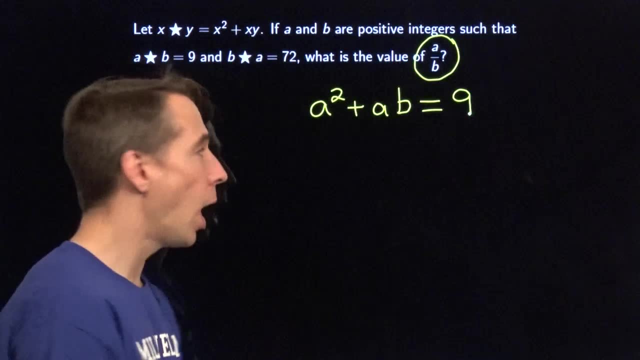 This b star a. Now b comes before the star. b is where the x is. We put b in for x over here. a is after the star. We put a in for y b star a is b squared plus b times a. 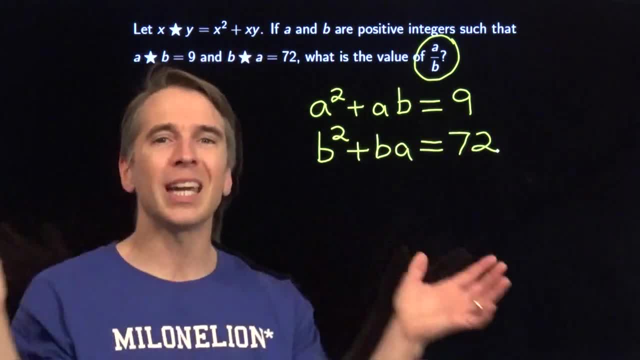 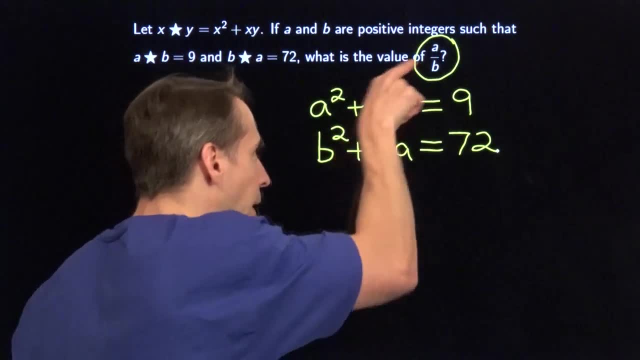 And we're told that that has to be 72. So we got rid of the stars And we have a couple of pretty messy equations to deal with. I'm going to keep our eye on the ball again. We see an. a all alone on the top, b- all alone on the bottom. 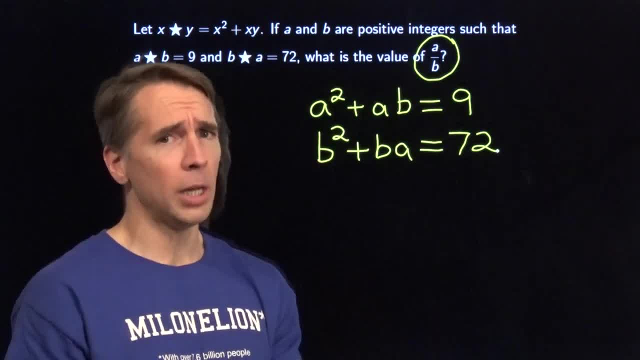 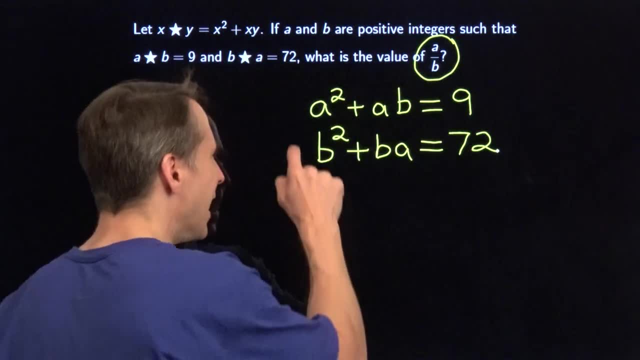 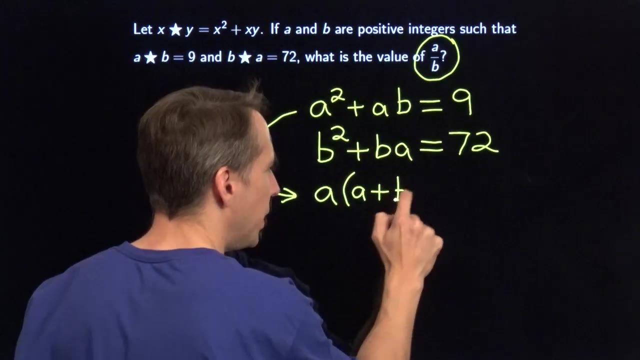 So we go looking for how to get an a all alone or a b all alone. I look at that first equation and I think: well, if I factor out an a, I get an a. that's kind of all alone. It's not quite all alone, because it's still multiplied by the a plus b that's left over when we factor it out. 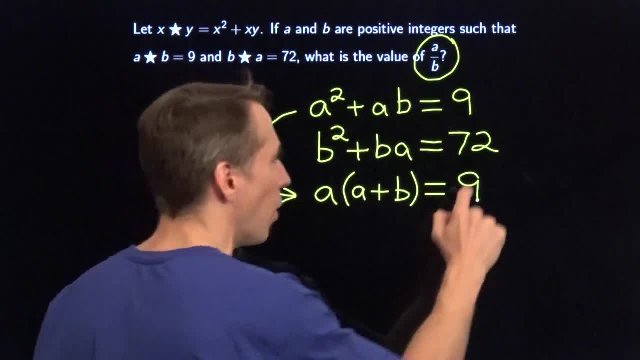 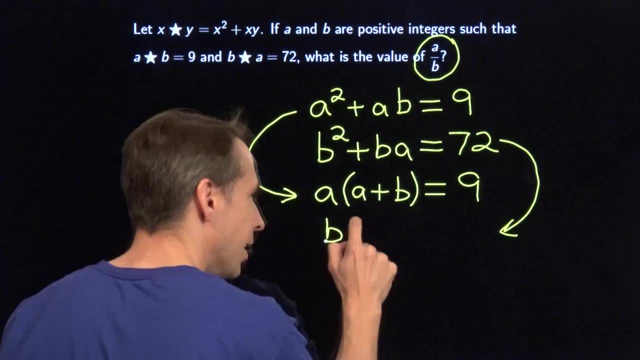 But I see I can kind of do something similar on the second equation as well. This time we're factoring out a- b. So I kind of have an a all alone here And I kind of have a b all alone down here. I factor out a b. 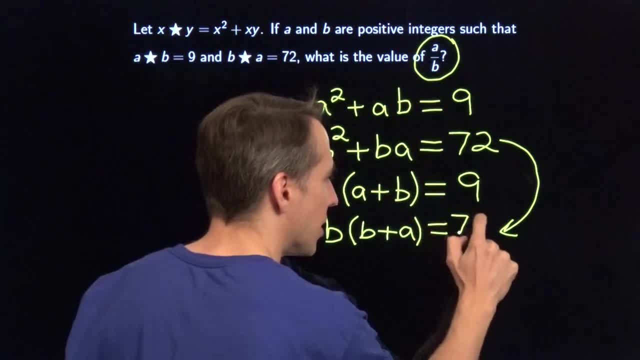 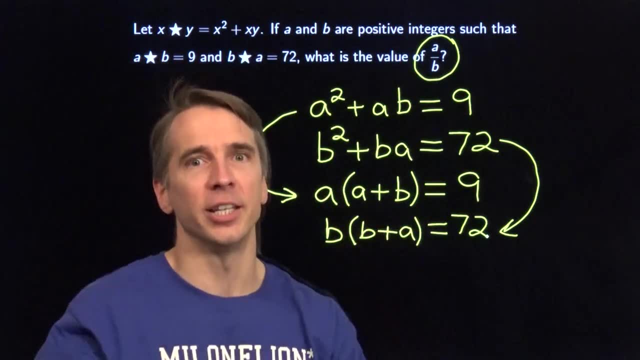 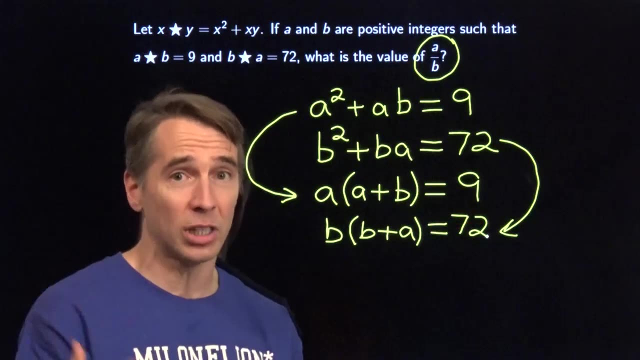 I have b times b plus a, And this has to equal 72. Now we see something really nice: a plus b and b plus a. They're the same, And we're keeping our eye on the ball. a over b. We want to divide this by this, because that will give us our a over b.